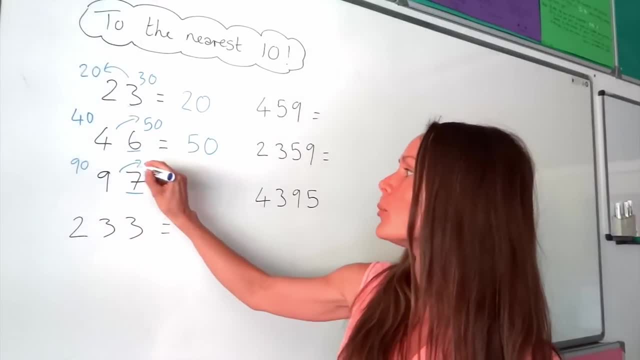 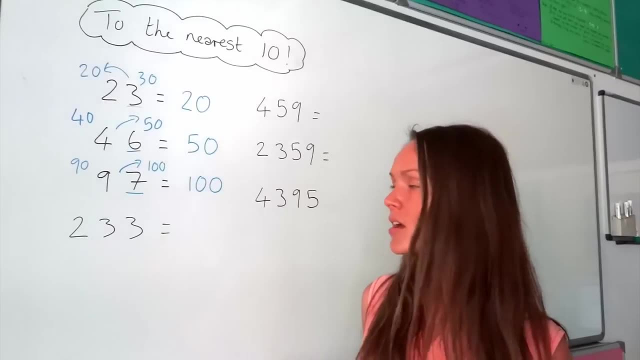 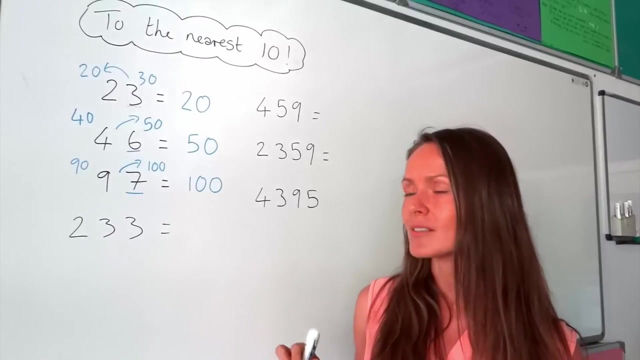 and because it's bigger than 5, it means we round up. so 100 is the answer. Now, just because the numbers are getting larger, now it doesn't matter. it's not getting more difficult. we're going to use exactly the same method. So I need to write down the two numbers in the 10 times table that are: 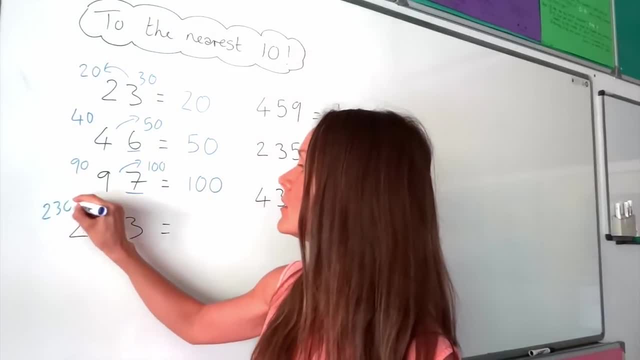 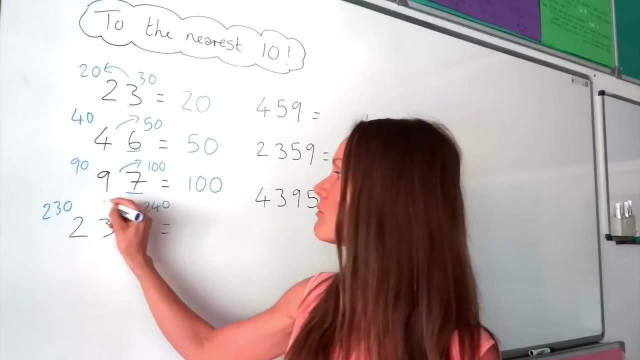 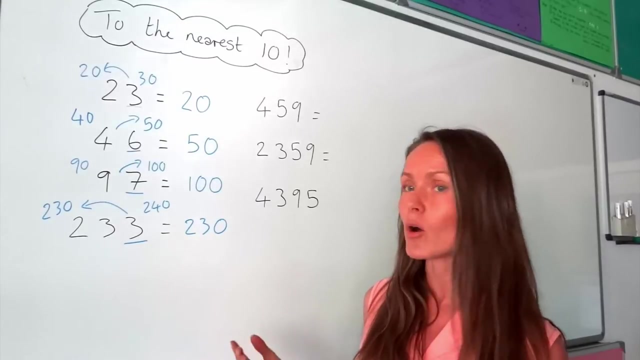 either side of this number here. so I've got 230 below And 240 above. So because the last digit is smaller than 5, it means you round down so it's just 230.. But, like I've said before, sometimes you might just be able to spot and you can see that that number 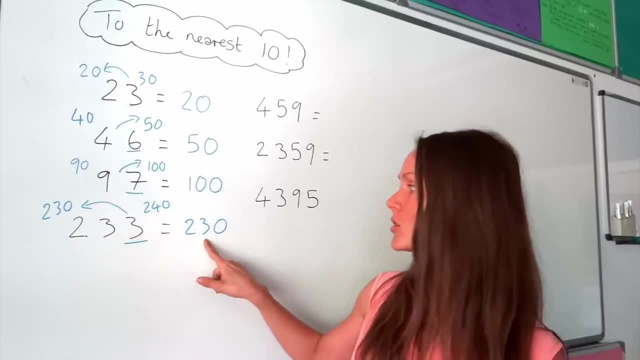 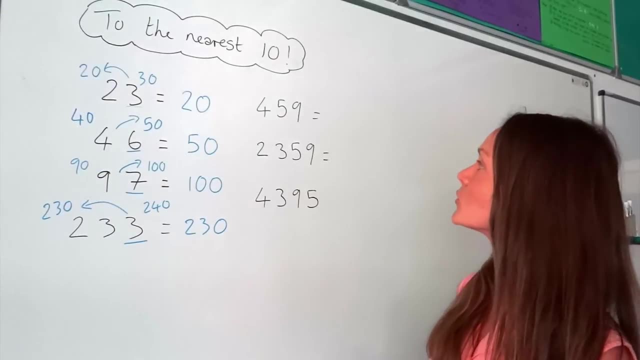 is just closer to 230, in which case you can just write that down straight away. You don't have to write out these numbers every time you do a rounding question. All right on to the top one. So again I'm going to write down the two numbers in the 10 times table that fall either side of 46. 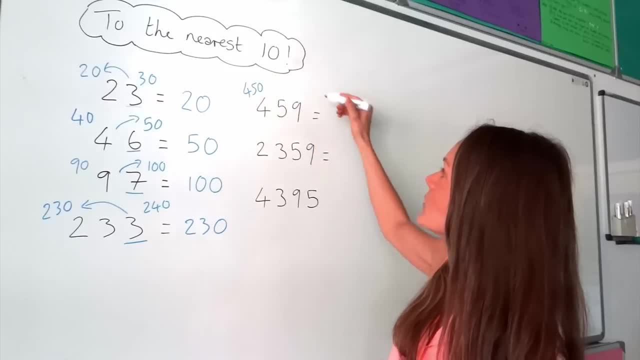 or the 10 times table. the one that's smaller than this number is 450 and the one that's bigger is 460, and because the last digit ends in a 9, we have to round up. so the answer is 460 and you can see that. 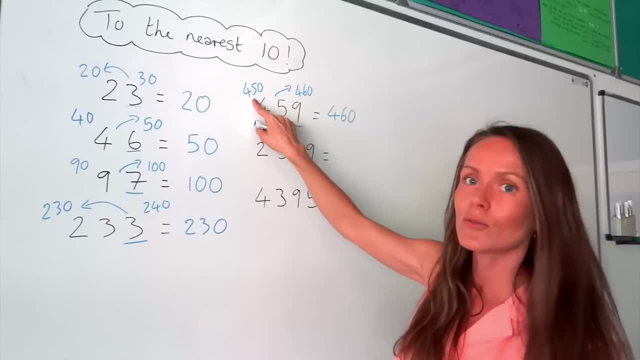 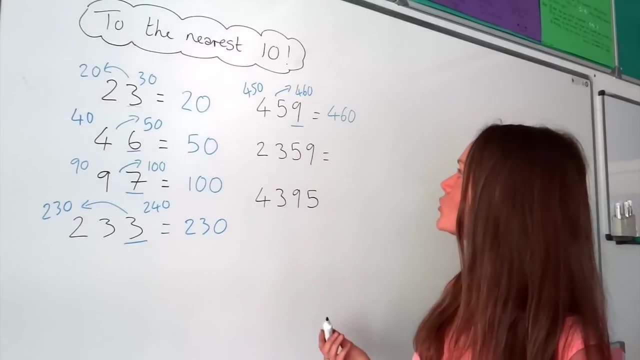 that number is much closer to 460 than it is to 450, so that makes sense. Now on to the thousand questions. So it's still the same method: write down the two numbers that are in the 10 times table, one that's smaller and one that's bigger. so for this one we're going to write down the two. 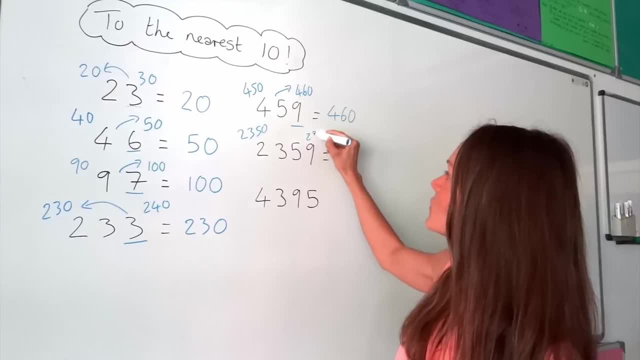 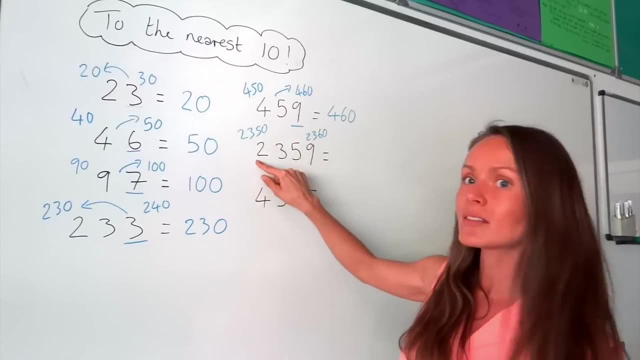 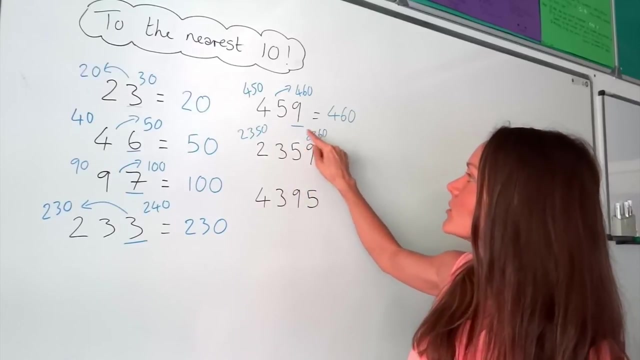 This one is 2350, and that one's 2360.. Now, if you're not sure how to get these, sometimes the smaller one is just this number here, except the 9 is always replaced with a 0. And this number over here is just 10 more than that one. 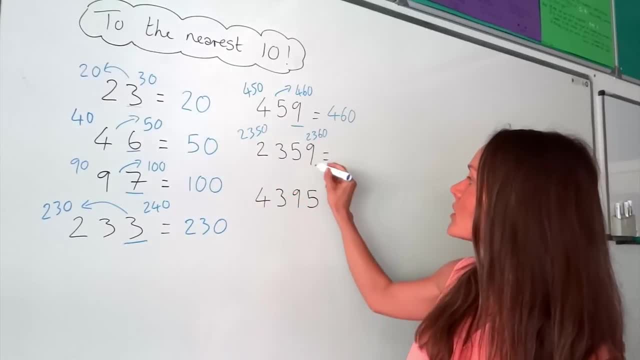 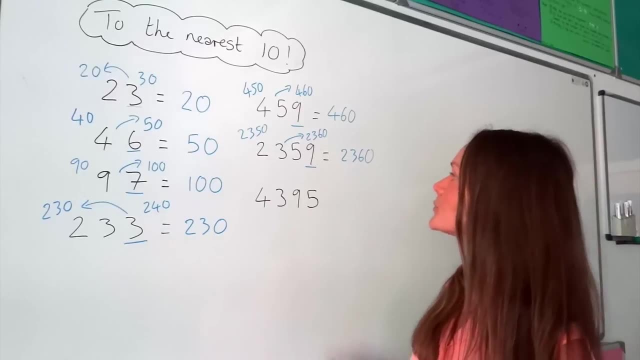 So if I add 10 to this one, it takes me to here, And because the last digit is a 9,, it means we're rounding up. So the answer is 2360.. Now for the final question, exactly the same to finish. 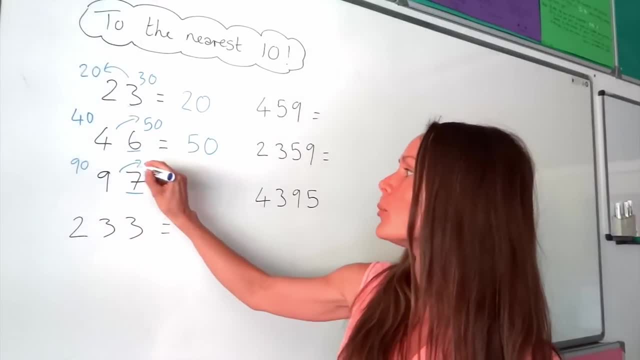 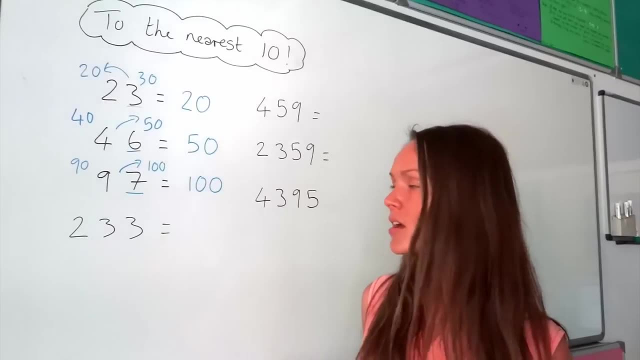 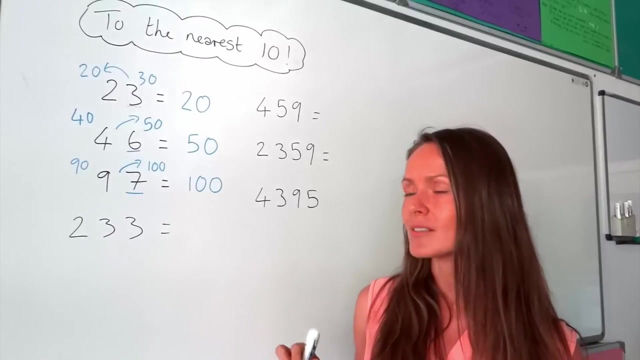 and because it's bigger than 5, it means we round up. so 100 is the answer. Now, just because the numbers are getting larger, now it doesn't matter. it's not getting more difficult. we're going to use exactly the same method. So I need to write down the two numbers in the 10 times table that are: 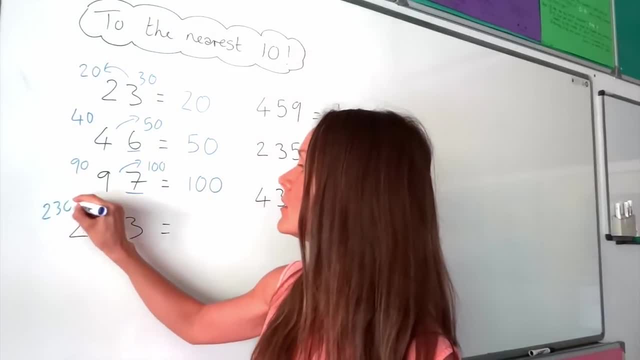 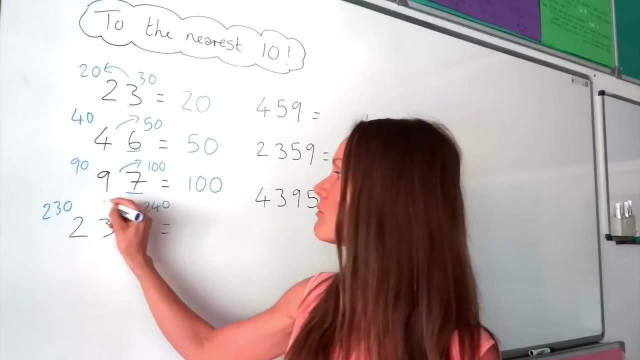 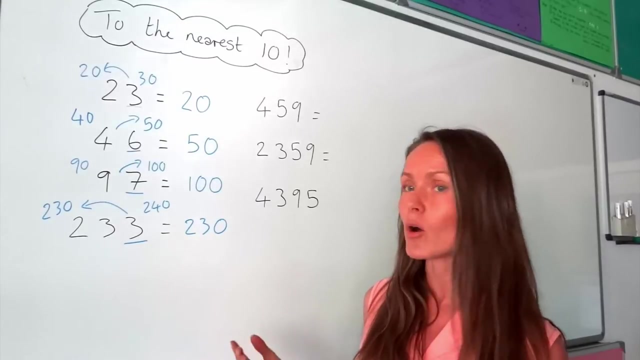 either side of this number here. so I've got 230 below And 240 above. So because the last digit is smaller than 5, it means you round down so it's just 230.. But, like I've said before, sometimes you might just be able to spot and you can see that that number 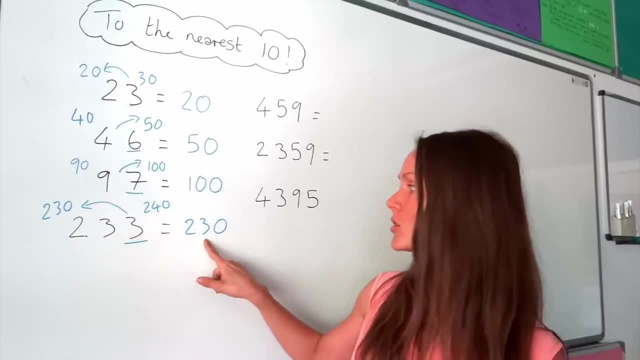 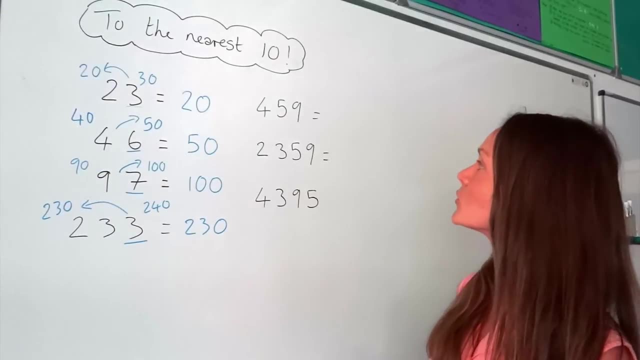 is just closer to 230, in which case you can just write that down straight away. You don't have to write out these numbers every time you do a rounding question. All right on to the top one. So again I'm going to write down the two numbers in the 10 times table that fall either side of 46. 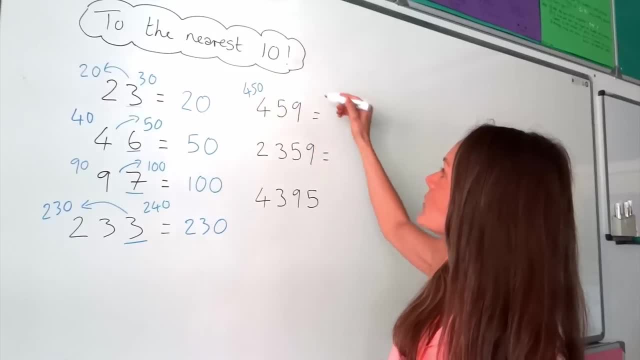 or the same number. So I'm going to write down the two numbers in the 10 times table. the one that's smaller than this number is 450 and the one that's bigger is 460, and because the last digit ends in a 9, we have to round up. so the answer is 460. 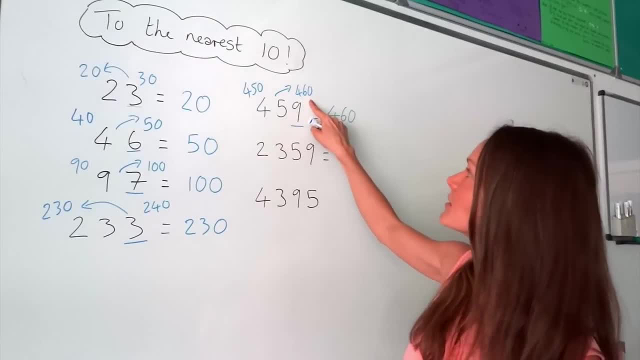 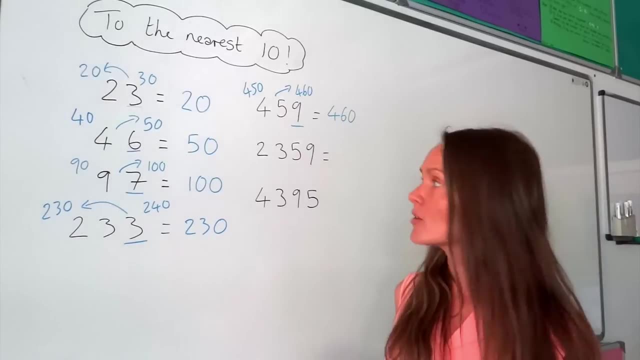 And you can see that that number is much closer to 460 than it is to 450. so that makes sense. Now on to the thousand questions. So it's still the same method. Write down the two numbers that are in the 10 times table, One that's smaller and one that's bigger. 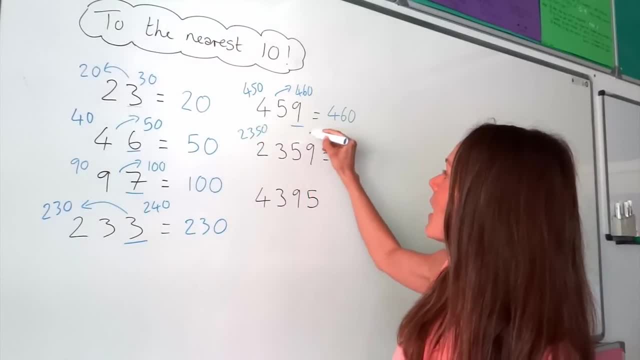 So for this one, I'm going to write down the two numbers in the 10 times table, and the one that's bigger and the one that's smaller, and one that's smaller one is 2350 and that one's 2360.. Now, if you're not sure how to get these, 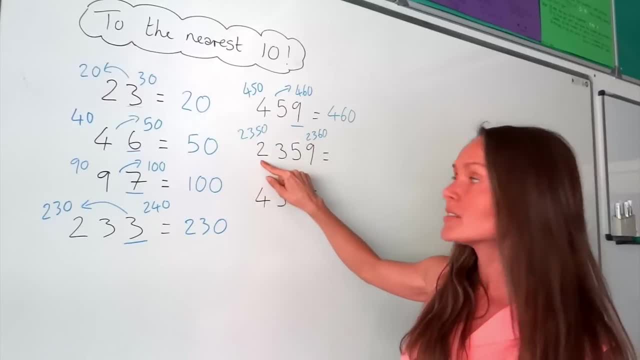 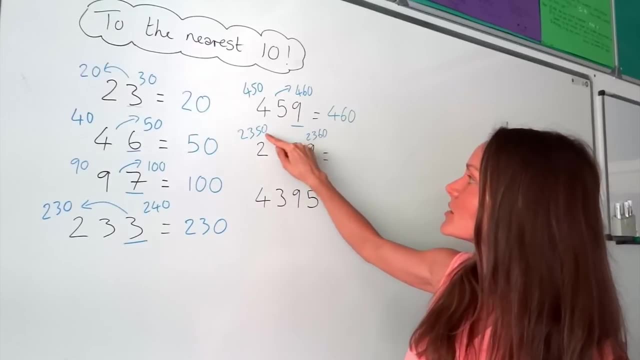 sometimes the smaller one is just this number here, except the 9 is always replaced with a 0, and this number over here is just 10, more than that one. so if I add 10 to this one, it takes me to here, and because the last digit is a 9, it 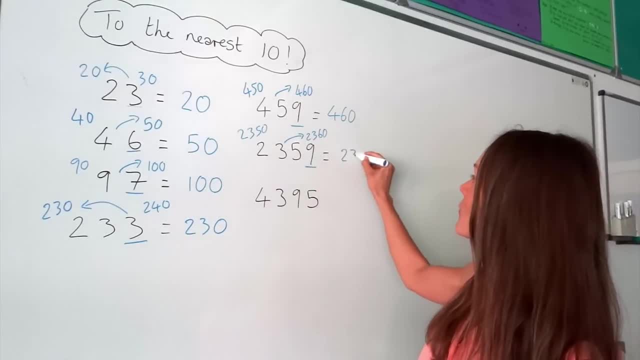 means we're rounding up, so the answer is 2360.. Now for the final question, exactly the same. to finish, write down the two numbers either side that are in the 10 times table. so remember: the smaller one is just this number, but replacing the 5 with a 0 and then the bigger one is just this number plus 10.